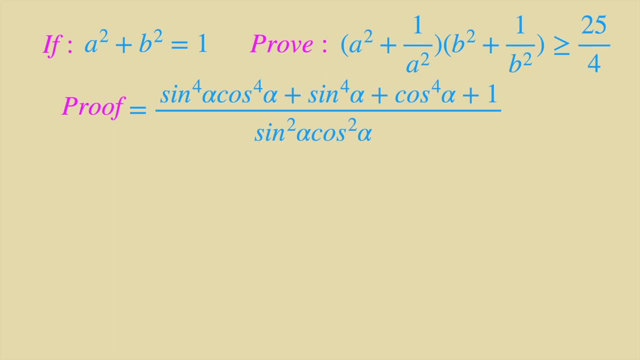 How to simplify it. We will do something with this part. We know: sine squared plus cosine squared equals 1. So sine squared plus cosine squared equals 1. And sine squared plus cosine squared- quantity squared still equals 1.. At the same time, there will be 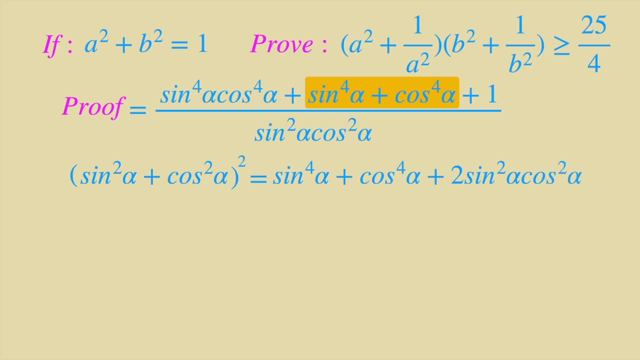 sine to the fourth and cosine to the fourth powers after squared. So we will get the expression of sine to the fourth plus cosine to the fourth. Substitute, the expression in The formula turns to be like this: At sign N times, cosine is only 1.. 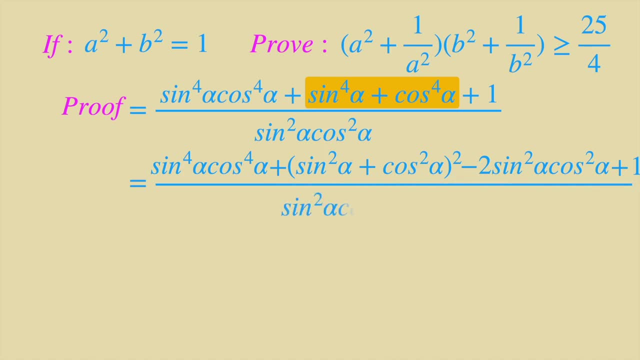 The formula turns out to be like this: Wow, it's getting more complicated, But don't worry. sine squared plus cosine squared equals 1.. Substitute 1 in it. the formula turns to be like this: Do you recognize that? That's the complete square formula. 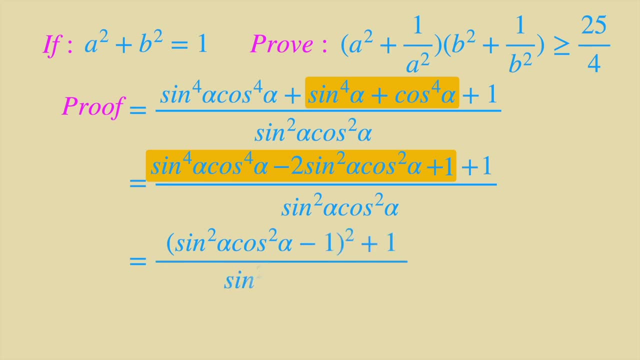 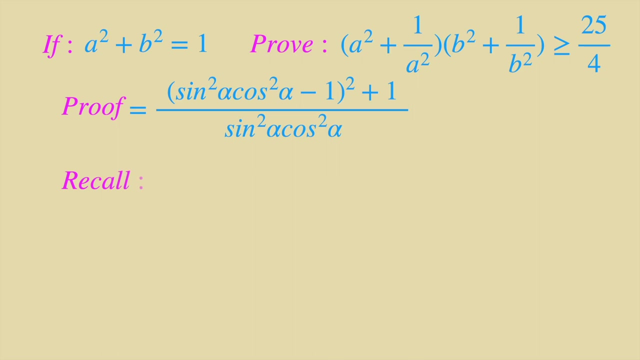 So we will have sine squared cosine squared minus 1, quantity squared plus 1 over sine squared cosine squared. Now we are close to the final answer, But before that there are still something to do with the formula. Recall sine alpha times cosine alpha equals one half times sine 2 alpha. 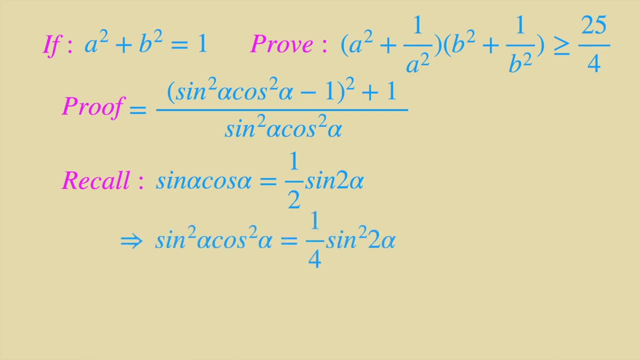 So sine squared alpha times cosine squared alpha equals one-fourth times sine squared of 2 alpha. Substitute that in, we will have this formula: Okay, There are one-fourths times sine squared 2 alpha in the numerator and denominator. Let it equal x. 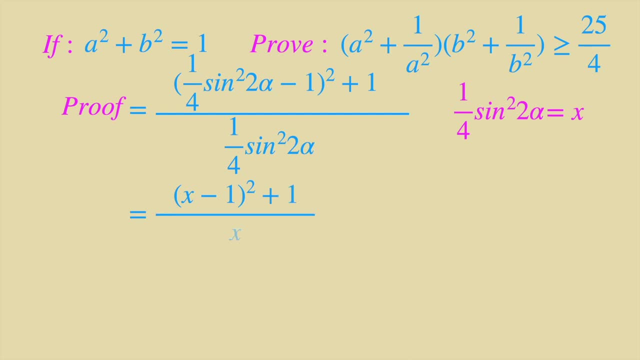 So the formula turns to be x minus 1, squared plus 1 over x, which simplifies to be x plus 2 over x minus 2.. We know sine squared 2 alpha is greater than 0 and is less than or equal to 1, so x is. 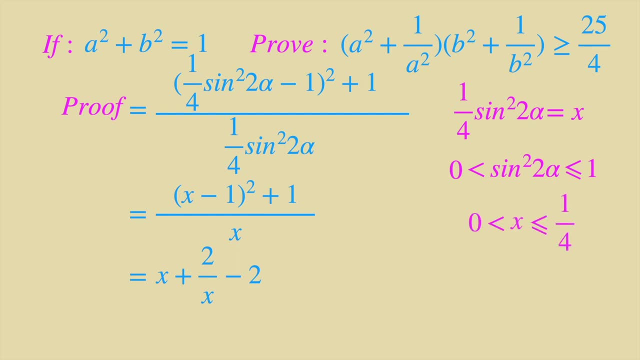 greater than 0.. and is less than or equal to one-fourth. Now we are close to the final answer. We want to prove this formula is greater than or equal to 25 over 4.. Where x is greater than 0 and is less than or equal to one-fourth.